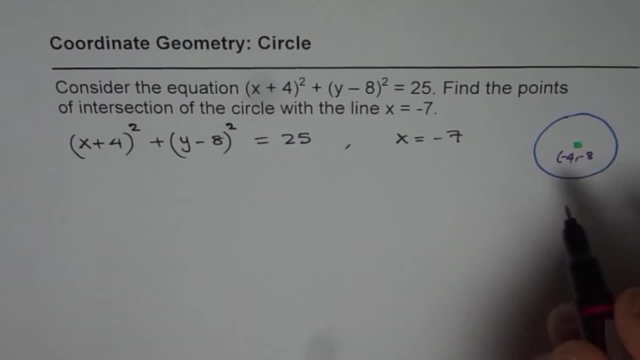 And the vertical line which you have is at minus 7, right. So minus 4 minus 9, is this point? So minus 7 is kind of line. going like this. This line is x equals to minus 7.. So we need to find these two points. 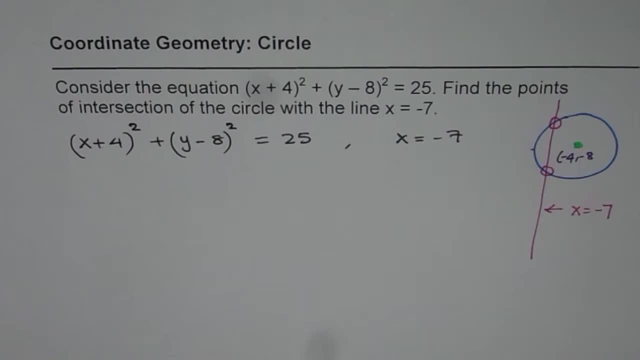 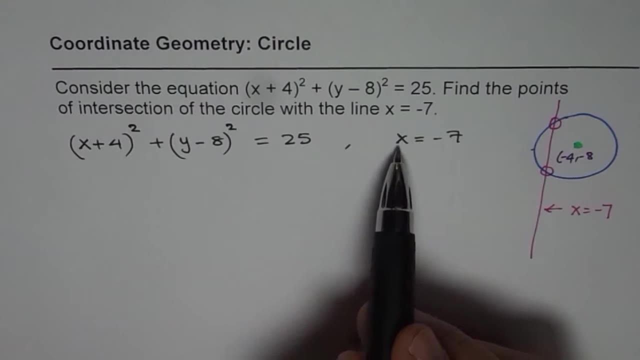 That's the whole idea. So how are you going to do it? You can pause the video, answer the question and then look into my suggestion. So what we do is we just substitute x equals to minus 7 in the equation and solve for y. okay, So let's substitute So we have minus. 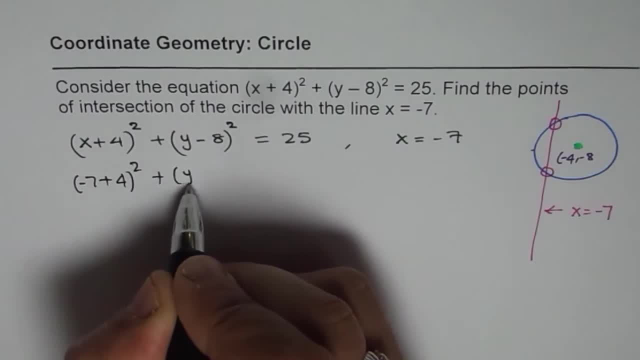 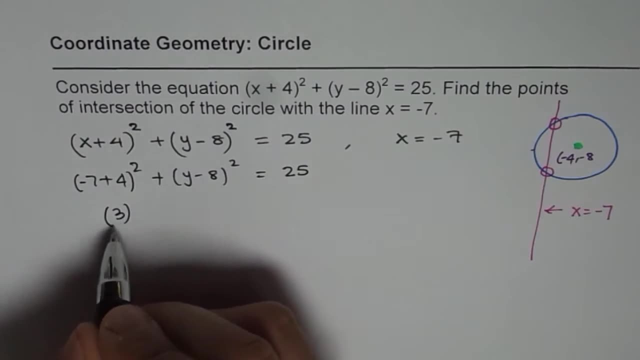 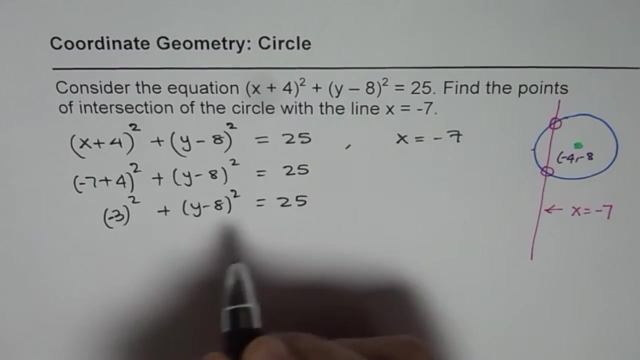 7 plus 4 whole square plus y minus 8 whole square equals to 25.. Now minus 7 plus 4 is 3.. Minus 3 square, Minus 3 square plus y minus 8 whole square equals to 25.. So we can bring this is 9.. 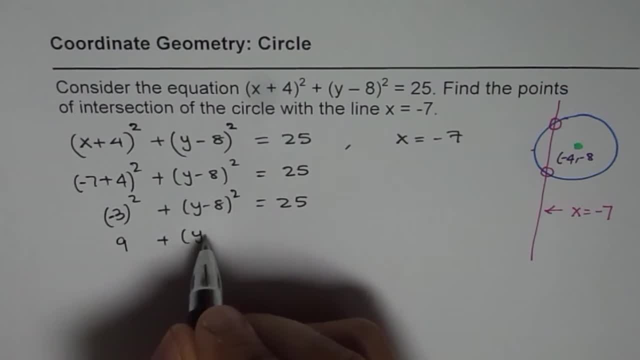 So we'll bring 9,. let me write here: 9 plus y minus 8 whole square equals to 25.. We say y minus 8 whole square equals to 25 minus 9, which is 16.. So we have y minus 8 equals. 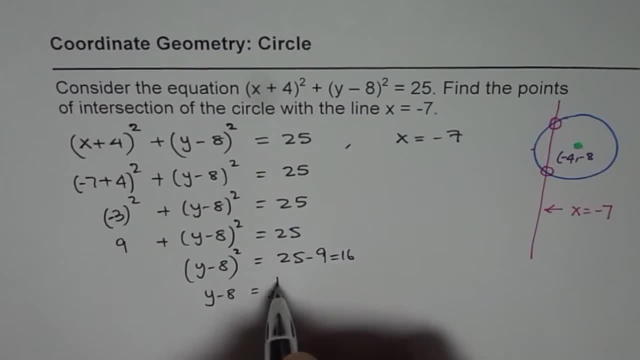 to square root of this, which is 16, square root of 16.. Now, remember, whenever you do square root, you should put plus and minus, since in this case, plus 4 square or minus 4 square, both are 16.. Do you see that? So you get plus and 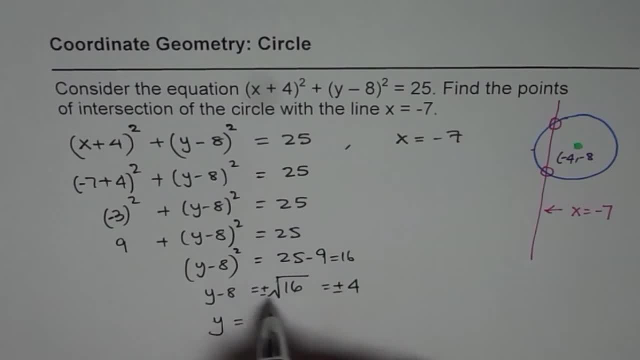 minus 4.. So y is equal to- let me take 8 to the side- 8 plus or minus 4.. So indeed, as expected, we do get two points. One is 8 plus 4.. So 8 plus 4 equals to 9 whole square plus. 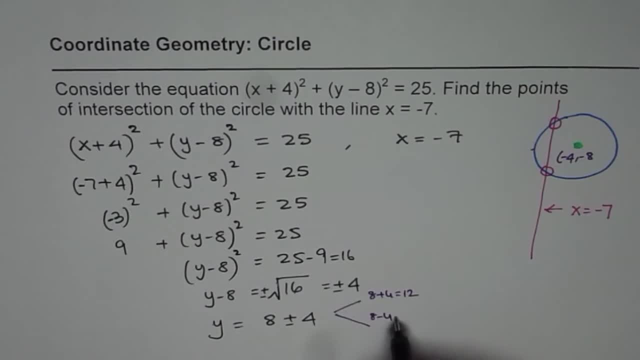 is 12 and 8 minus 4 will be 4.. So our answer here is that the two points are: x value is minus 7,, right x value is minus 7, y value could be 4 or 12.. So the points of intersection. 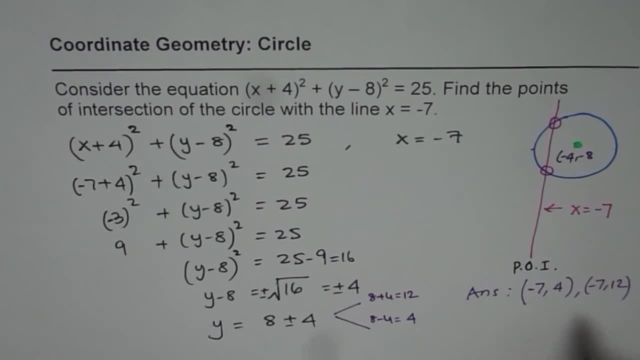 are. let me write points of intersection. are these right? So that is how the question should be solved. I hope you understand and appreciate it. Thank you and all the best.